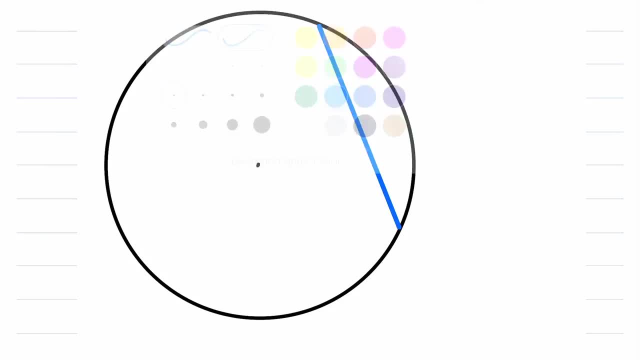 so that I can go eat Here. we have a chord of the circle. Remember that a chord is a line segment whose endpoints both lie on the circle. So that's great. This is a chord. How do we find its length? Well, there are really two key pieces of information that 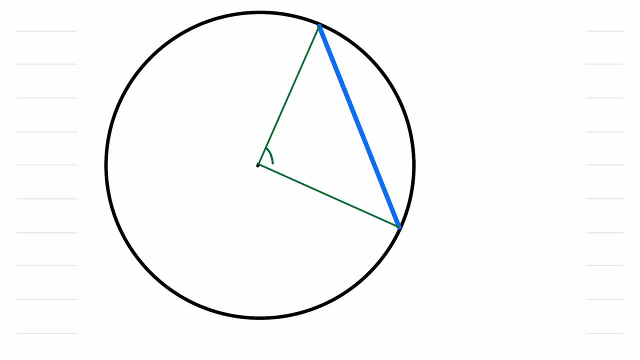 we need to know to find the length of this chord, We need to know the measure of the central angle subtended by the chord, That's this angle- here We'll call this angle theta- And we need to know the measure of the radius of the circle. 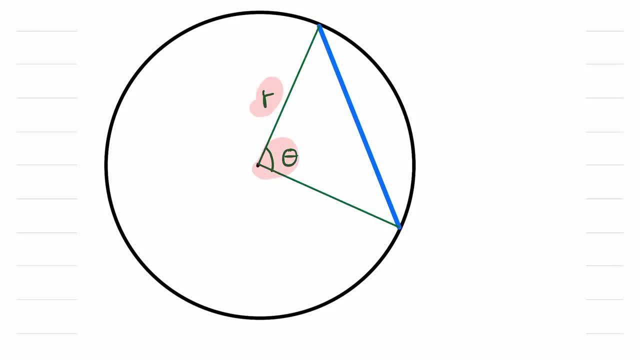 We will call that r. Alright. now how will we use this information to find the length of this chord? Well, it's all about triangles. The first thing we do is drop a perpendicular line segment from the center of the circle to the chord, So something like that Again. 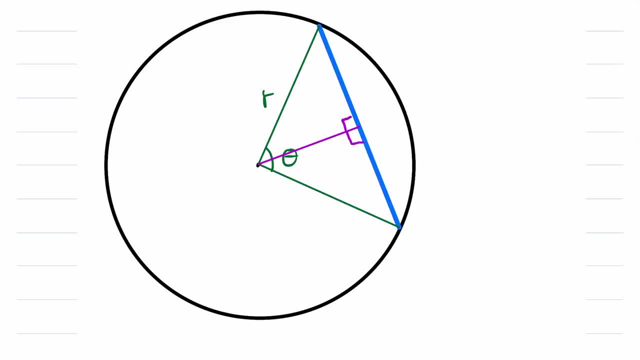 this is a perpendicular line segment, so it'll indicate that both of these angles are right angles. If you haven't tried figuring out the formula for chord length by yourself, I definitely recommend giving it a go. Try picking it up from here. Alright, now we will carry on and go the rest of the way. Notice that these two right 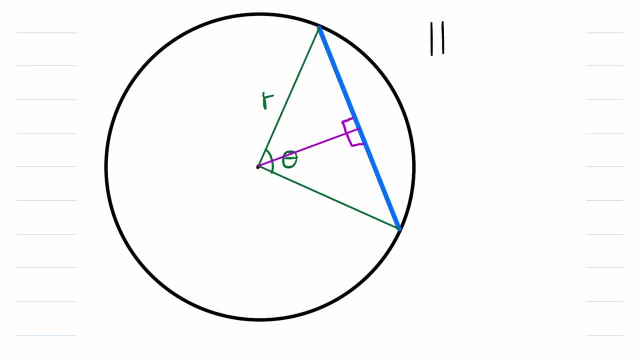 triangles are congruent. How do we know that? We know it because of the hypotenuse leg triangle congruence postulate, often abbreviated HL. We know that the hypotenuses of these two right triangles are congruent because they are both radii of the same circle. And then 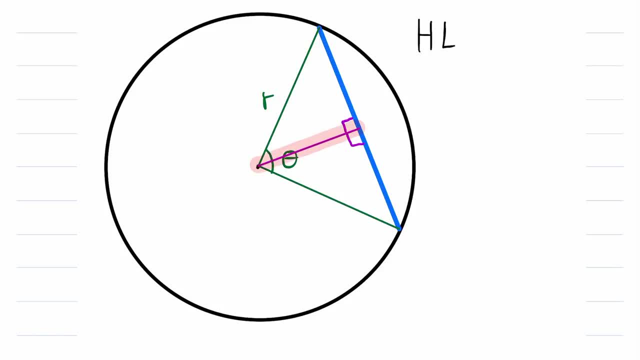 this line segment. here is a leg of both of the right triangles And of course it's congruent to itself. So we have congruent hypotenuses, we have a congruent leg. these are both right triangles. so by the hypotenuse leg congruence postulate, they are congruent right triangles. 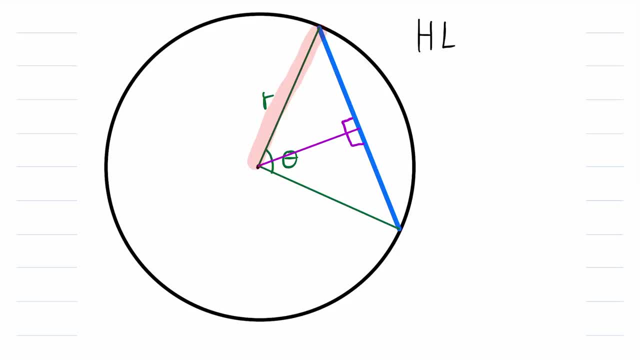 So these right triangles are congruent. We know that this side matches this side, this side matches itself. so that means this side of this right triangle must be congruent to this side of this right triangle. So that means if the length of the whole chord is x, then the length of this piece has to. 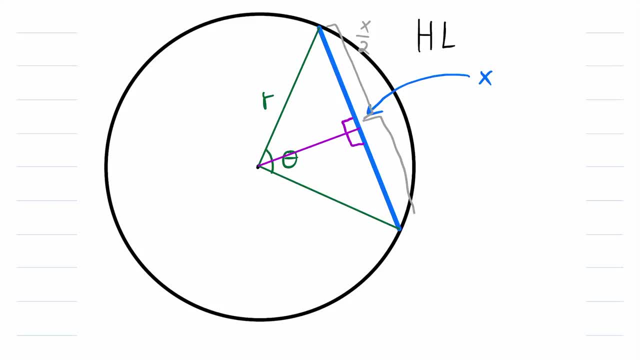 be x over 2, and the length of this piece has to be x over 2 as well, Because these two pieces have to be equal and together they have to add up to the whole chord length, which, again, we're calling x. So if we can find the length of this leg of either right, 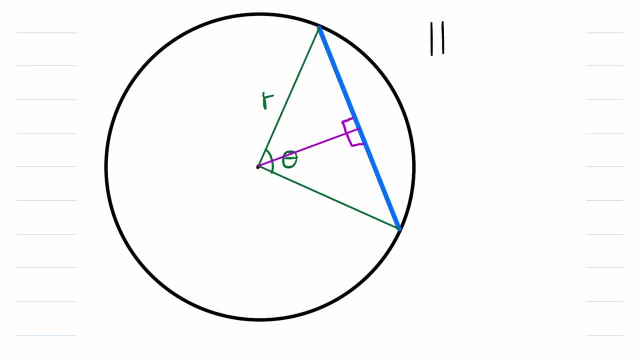 triangles are congruent. How do we know that? We know it because of the hypotenuse leg triangle congruence postulate, often abbreviated HL. We know that the hypotenuses of these two right triangles are congruent because they are both radii of the same circle. And then 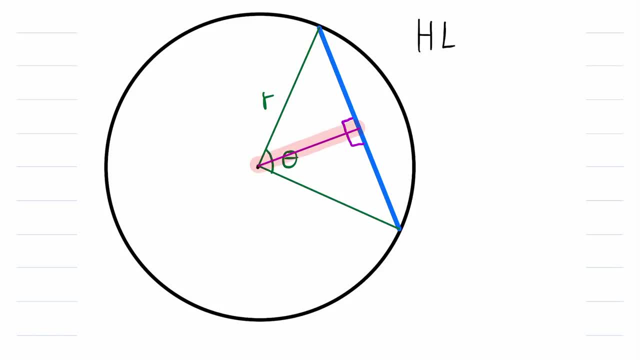 this line segment. here is a leg of both of the right triangles and of course it's congruent to itself. So we have congruent hypotenuses, we have a congruent leg. these are both right triangles. so by the hypotenuse leg congruence postulate, they are congruent right triangles. 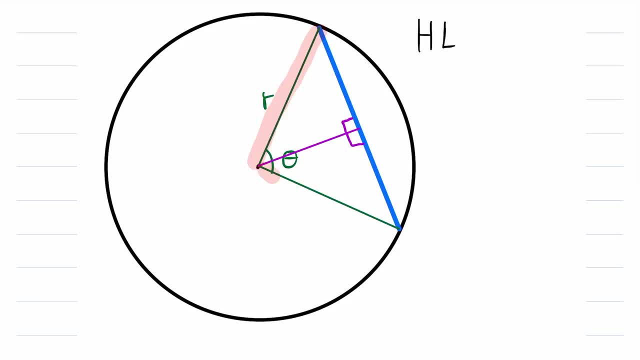 So these right triangles are congruent. We know that this side matches this side, this side matches itself. so that means this side of this right triangle must be congruent to this side of this right triangle. So that means if the length of the whole chord is x, then the length of this piece has to. 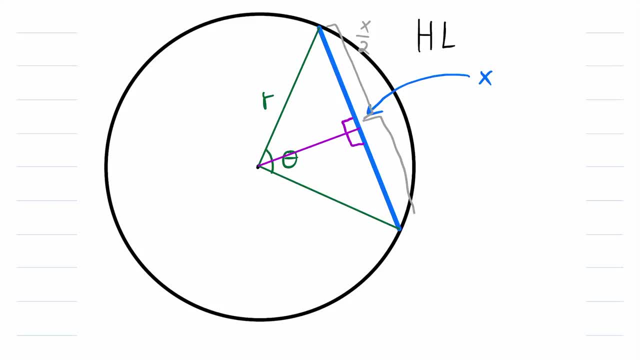 be x over 2, and the length of this piece has to be x over 2 as well, because these two pieces have to be equal and together they have to add up to the whole chord length, which, again, we're calling x. So if we can find the length of this leg of either right, 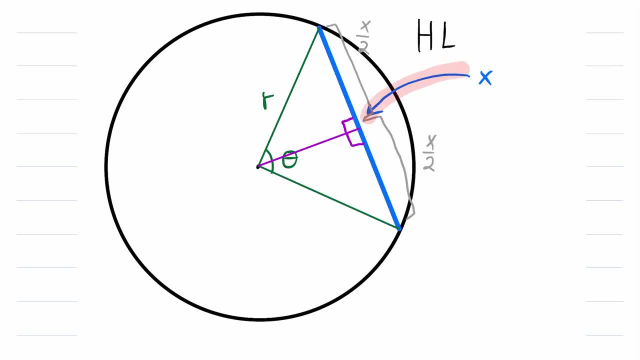 triangle. all we have to do is double it to find the total chord length. Now notice that this bigger triangle is an isosceles triangle because these two sides are congruent, because they're both radii of the same circle. Then, by the isosceles triangle theorem, the angles 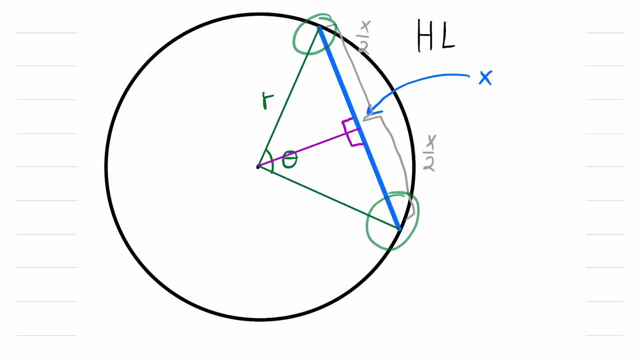 opposite, the congruent sides are also congruent. So this angle over here is congruent to this angle right over here. Then, going back to our right triangles, remember we already know that these triangles are congruent. so we know there are three pairs of congruent angles. 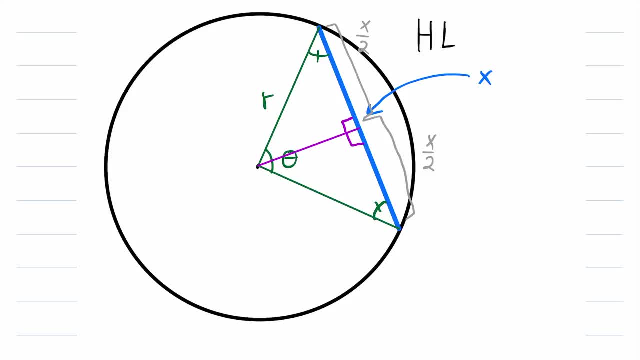 between them, but now we know exactly which pairs of angles are congruent. We know this angle is congruent to this angle. we know this angle is congruent to this angle. therefore, this angle that I'm marking in pink is congruent to this angle. So now this is just like the 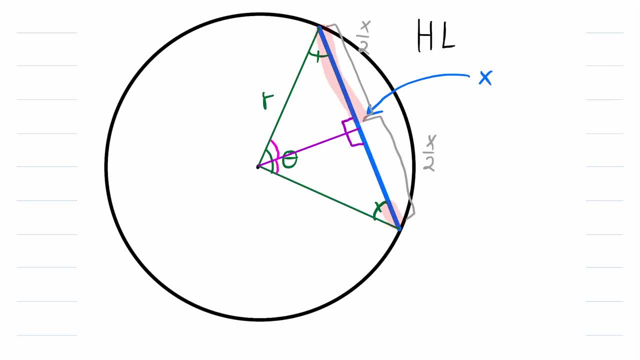 situation we had with the chord and these two legs of the right triangles. We had two congruent segments that had to add up to a measure of x, so the measure of each segment had to be x over 2.. And now, since these two angles have to add up to theta and the two angles have the same, 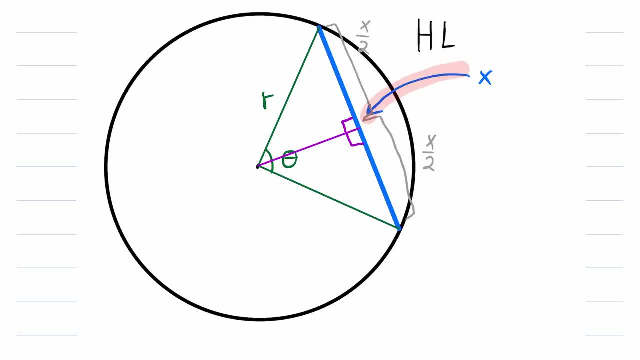 triangle. all we have to do is double it to find the total chord length. Now notice: this bigger triangle is an isosceles triangle, because these two sides are congruent, because they're both radii of the same circle. Then, by the isosceles triangle theorem, the angles 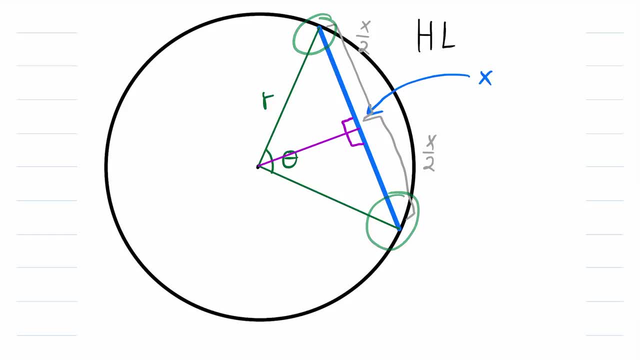 opposite, the congruent sides are also congruent. So this angle over here is congruent to this angle right over here. Then, going back to our right triangles, remember we already know that these triangles are congruent. So we know there are three pairs of congruent angles. 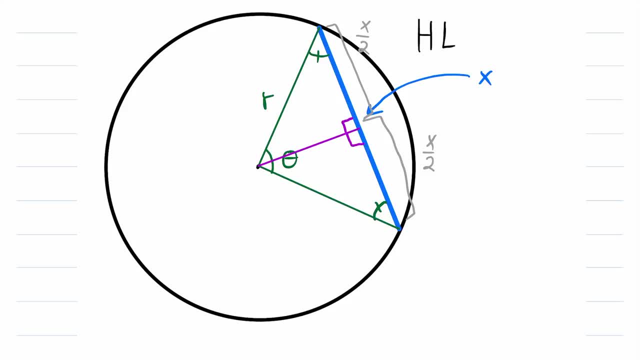 between them, but now we know exactly which pairs of angles are congruent. We know this angle is congruent to this angle. we know this angle is congruent to this angle. therefore, this angle that I'm marking in pink is congruent to this angle. So now this is just like the 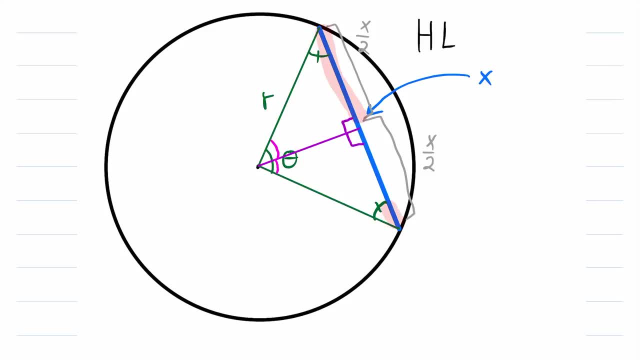 situation we had with the chord and these two legs of the right triangles. We had two congruent segments that had to add up to a measure of x, so the measure of each segment had to be x over 2.. And now, since these two angles have to add up to theta and the two angles have the same, 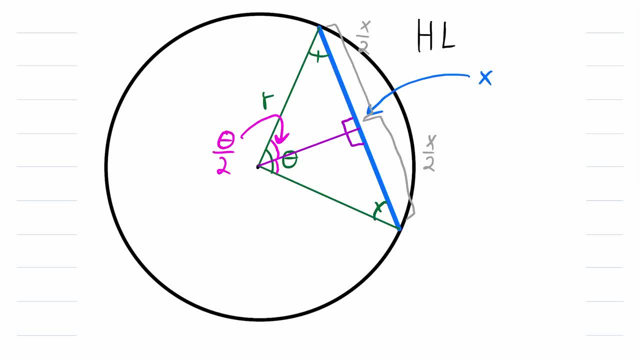 measure. each angle has to have a measure of theta over 2.. So each one of these pink angles has a measure of theta over 2, and together they make up this angle that has a measure of theta. So now that we know the measure of this angle in this right triangle, 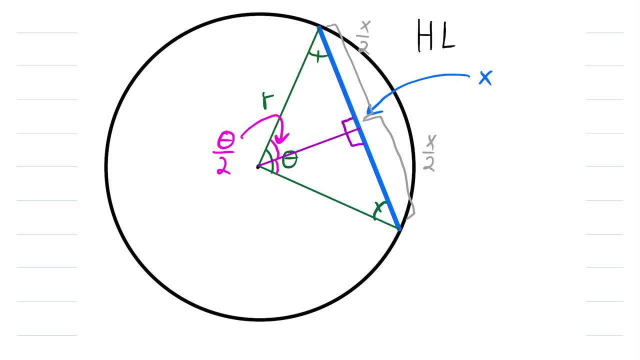 we can start to use trigonometric ratios. But which ratio should we use? Sine, cosine or tangent? This is the angle that we know. We want to find the length of the side opposite this angle and we know that the hypotenuse has a measure of r, So we want to use the sine. 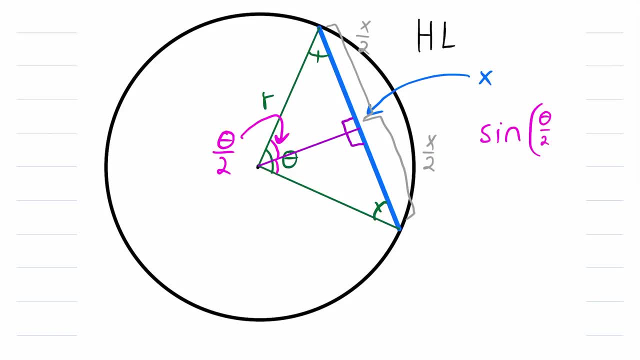 ratio, because the sine of theta over 2, the measure of this angle is going to be equal to the ratio of the opposite side, which we know has a measure of x divided by 2, divided by the measure of the hypotenuse, which is r, the radius length. 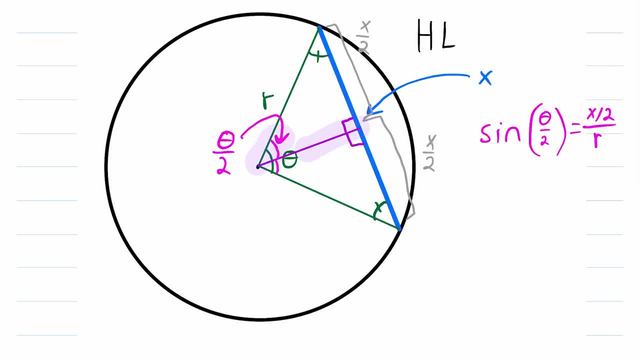 Because, remember, the sine of an acute angle in a right triangle is equal to the ratio of the opposite side over the hypotenuse. So x over 2 is the measure of the opposite side and r is the measure of the hypotenuse. 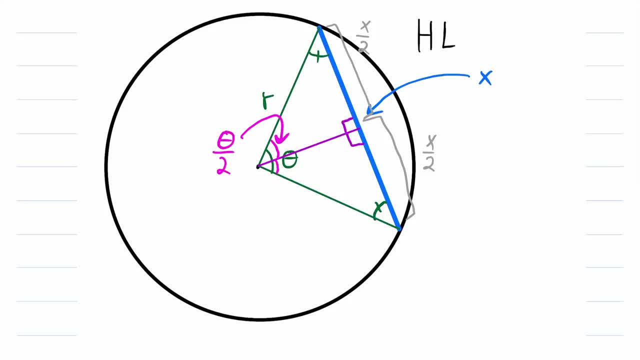 measure. each angle has to have a measure of theta over 2.. So each one of these pink angles has a measure of theta over 2, and together they make up this angle that has a measure of theta. So now that we know the measure of this angle in this right triangle, 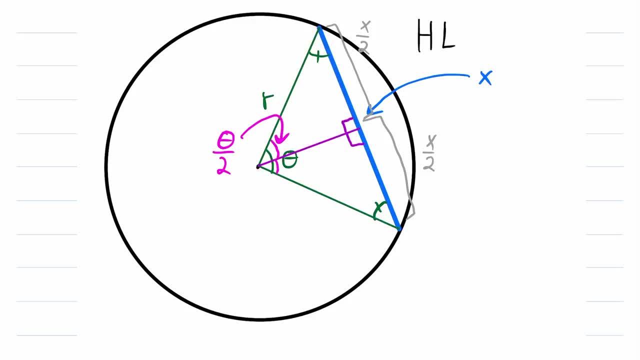 we can start to use trigonometric ratios, But which ratio should we use? Sine, cosine or tangent? Well, this is the acute angle. This is the angle that we know. We want to find the length of the side opposite this. 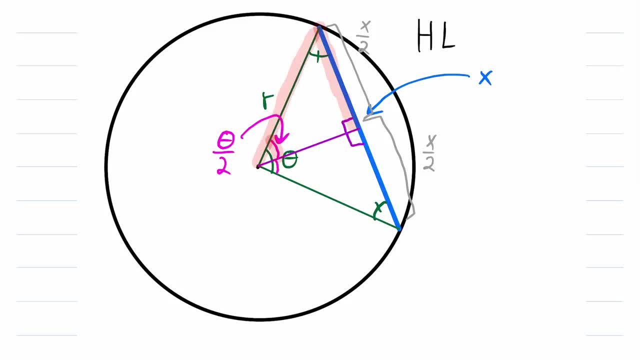 angle and we know that the hypotenuse has a measure of r. So we want to use the sine ratio, because the sine of theta over 2, the measure of this angle is going to be equal to the ratio of the opposite side, which we know has a measure of x divided by 2, divided 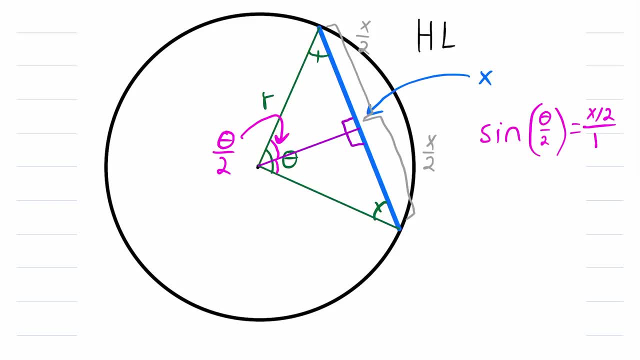 by the measure of the hypotenuse, which is r, the radius length, Because, remember, the sine of an acute angle in a right triangle is equal to the ratio of the opposite side over the hypotenuse. So x over 2 is the measure of the opposite. 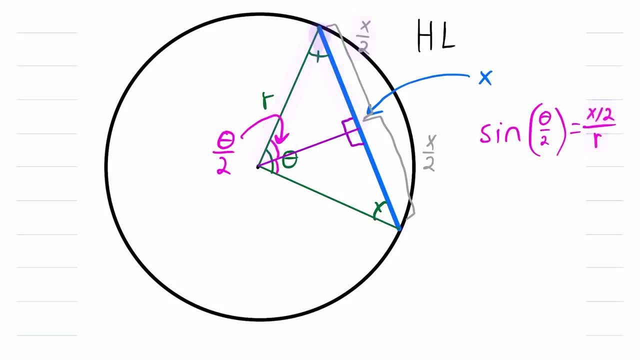 side and r is the measure of the hypotenuse. So now this is cake. we've basically got our formula. Remember what we're trying to find: the length of a chord, which has a measure of x. So in this formula we just have to solve: 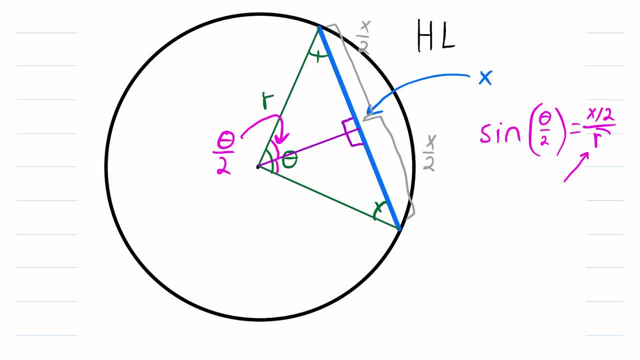 for x by r in order to get rid of that division by r, Then what we have left on this side is x over 2, and that's equal to this side multiplied by r. That's sine of theta over 2 multiplied by r. Now, 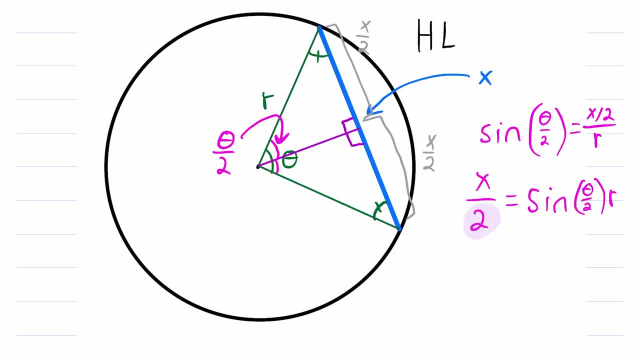 to finish getting x by itself, we just have to multiply both sides by 2 to get rid of the division by 2.. So that leaves us with x as desired and that's equal to this side multiplied by 2.. I'm going to write that as 2 times r, times sine of theta over 2.. Remember that it doesn't matter. 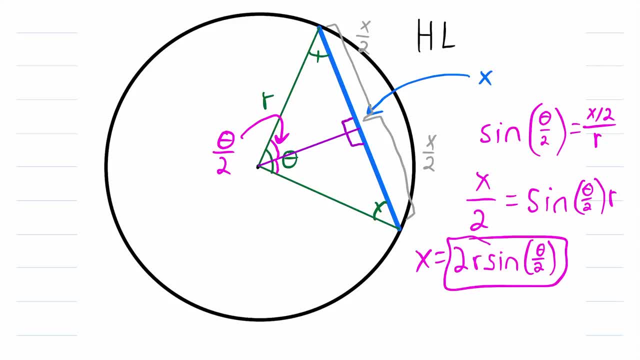 what order we multiply things in, so I just write it in this order so that it looks nicer. So that's it. That's how you find the length of a chord. If you have a chord in a circle with radius length r and the central angle subtended by the chord has an angle measure of theta, then to find the chord 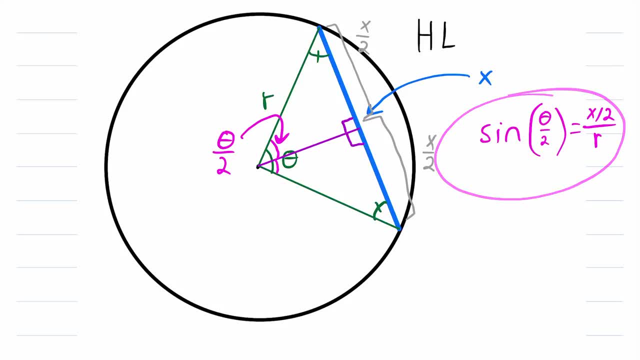 So now we've got our formula. Remember what were trying to find? the length of this chord which has a measure of x. So in this formula we just have to solve for x. So what we'll do first is multiply both sides. 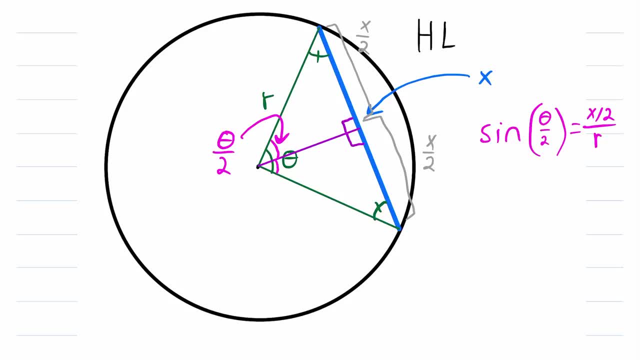 by r in order to get rid of that division by r. Then what we have left on this side is x over 2, and that's equal to this side multiplied by r. That's sine of theta over 2 multiplied by r. Now, to finish getting x by itself, we just have to multiply both sides by 2 to get rid of the division. 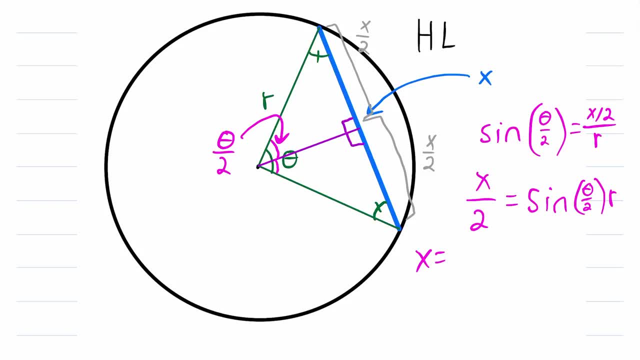 by 2.. So that leaves us with x as desired, and that's equal to this side multiplied by 2.. I'm going to write that as 2 times r, times sine of theta over 2.. Remember that it doesn't matter what order we multiply things in, so I just write it in this order so that it looks nicer. So that's. 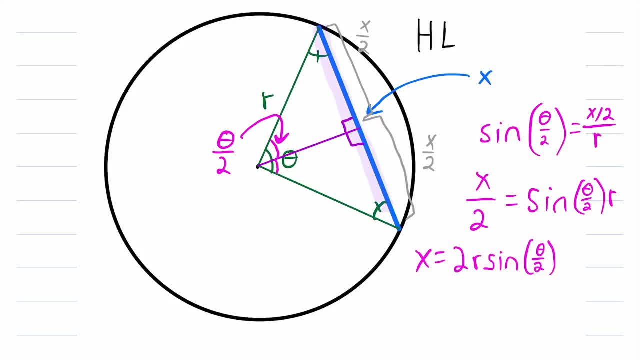 it. That's how you find the length of a chord. If you have a chord in a circle with radius length r and the central angle subtended by the chord has an angle measure of theta, then to find the chord length you just multiply 2 times the length of the radius r, times the. 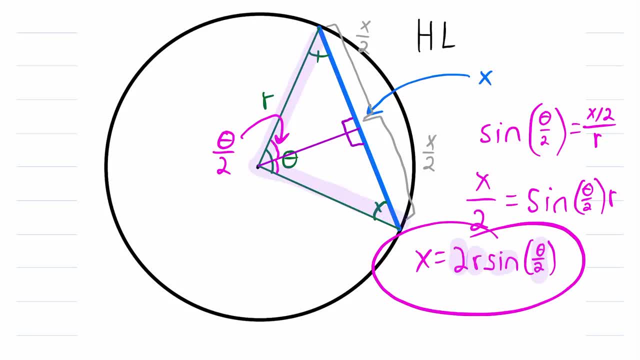 sine of theta over 2.. So that's it. That's how you find the length of a chord. If you have a sine of the measure of the central angle divided by 2, which is theta over 2, and it doesn't matter. 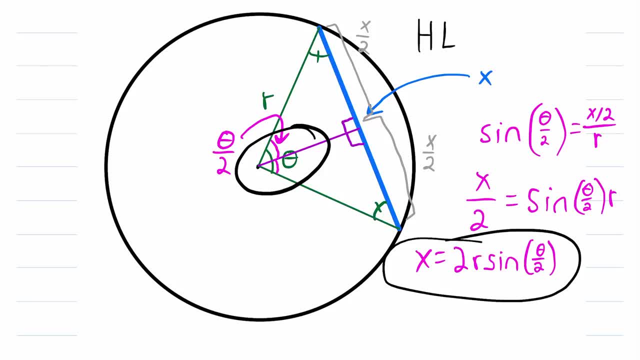 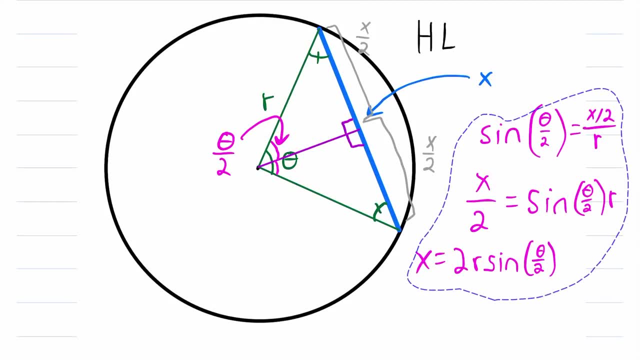 if theta is in degrees or radians, You still use the same formula. just make sure that your sine calculation is in the right units. Alright, now let me move all of this pink writing up and let's quickly do an example before we go. Let's say that the radius length r is equal to 10. 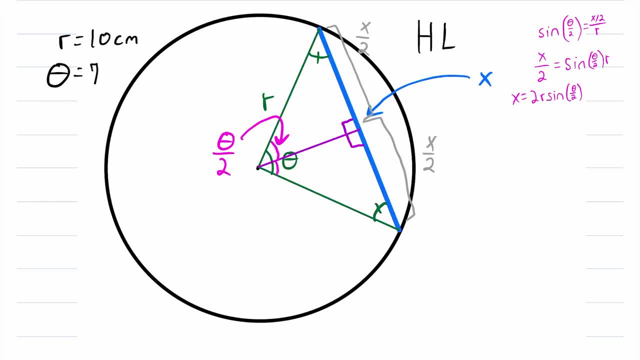 centimeters, and we'll say that theta is equal to 70 degrees. So then, what's the length of the chord? Well, we just have to use our handy-dandy formula. So the chord length x is equal to 2 times the radius length, which, remember, is 10 centimeters. and then that's. 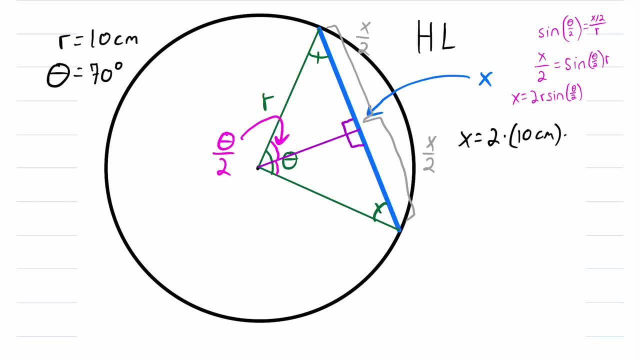 getting multiplied by sine of theta over 2.. So in this case that's just sine of 70 degrees over 2, which I know is sine of 35 degrees. 70 over 2 is 35. And this is equal to about 11.48 centimeters. 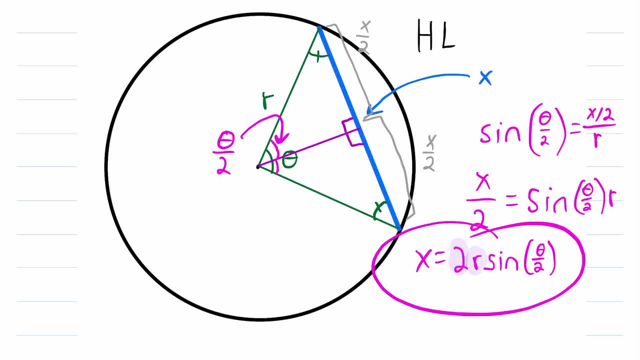 length. you just multiply 2 times the length of the radius, r times the sine of theta over 2.. That's the sine of the measure of the central angle divided by 2, which is theta over 2.. And it doesn't matter if theta is in degrees or radians. You still use the same formula, just make sure. 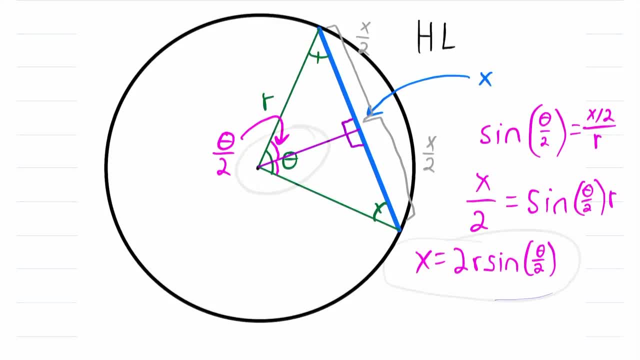 that your sine calculation is in the right units. Alright, now let me move all of this pink writing up and let's quickly do an example before we go. Let's say that the radius length r is equal to 10 centimeters, and we'll say that theta is equal to 70 degrees. So then, what's the? 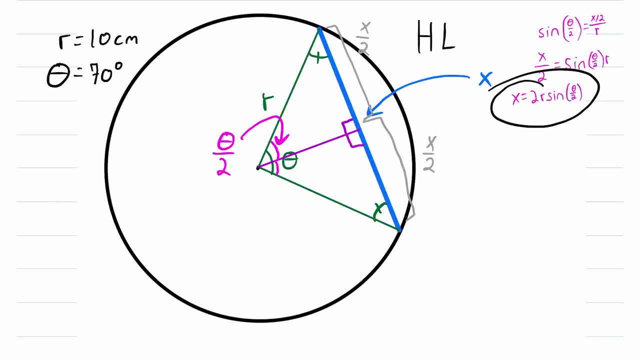 length of the chord. Well, we just have to use our handy-dandy formula. So the chord length x is equal to 2 times the radius length, which, remember, is 10 centimeters, and then that's getting multiplied by sine of theta over 2.. So in this case, that's just sine of 70 degrees over 2, which 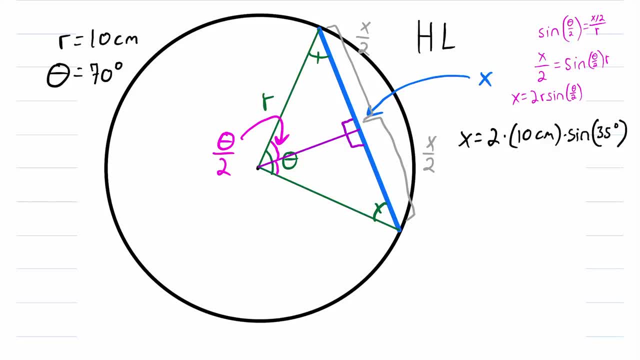 I know is sine of 35 degrees. 70 over 2 is 35. And this is equal to about 11.48 centimeters. So if this radius is 10 centimeters and this angle is 70 degrees, then this chord length is: 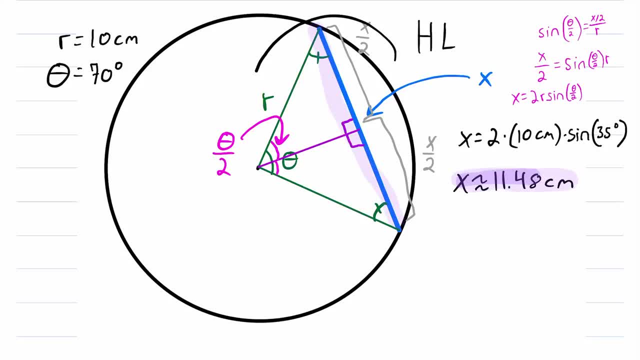 about 11.48 centimeters. So that's how you find the length of a chord and why this splendid formula works. Let me make that formula nice and big before we go. x equals 2r sine of theta over 2.. So I hope this video helped you understand how to find the length of a chord. Let me know in. 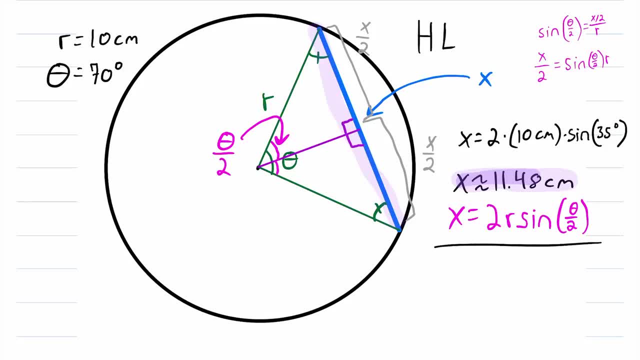 the comments if you have any questions, need anything clarified or of any other video requests. Thank you very much for watching and I'll see you in the next video. Bye, Thanks for watching. I'll see you next time and be sure to subscribe for the swankiest. 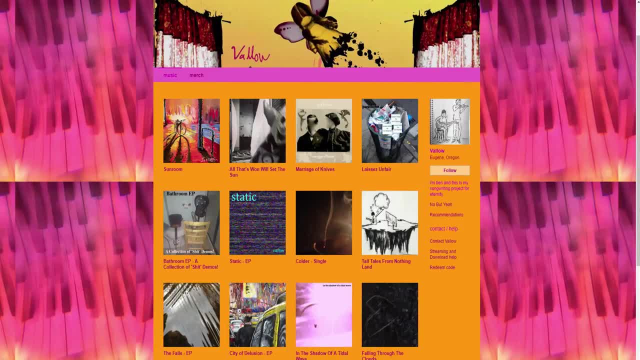 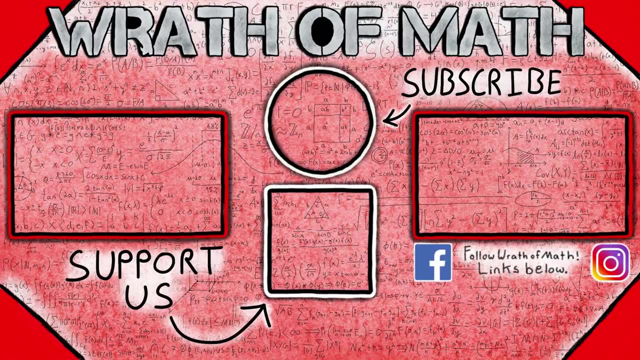 math lessons on the internet. And a big thanks to Valo who, upon my request, kindly gave me permission to use his music in my math lessons. Link to his music in the description. Thanks for watching and I'll see you in the next video.